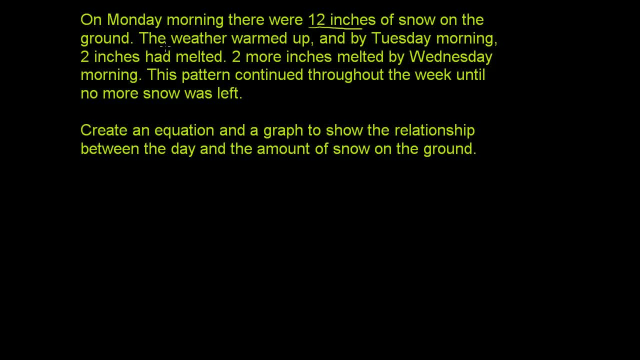 On Monday morning there were 12 inches of snow on the ground. The weather warmed up and by Tuesday morning 2 inches had melted. All right, so we'll have 10 left, 2 more inches melted by Wednesday morning. 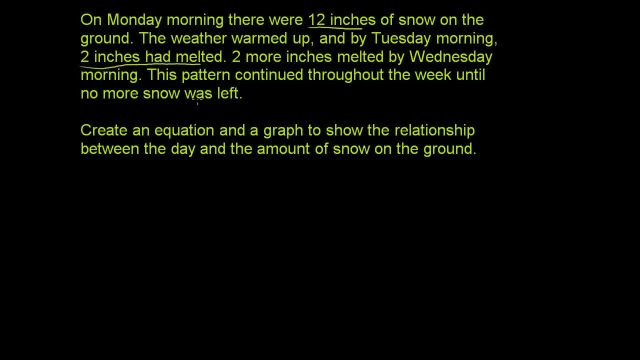 This pattern continued throughout the week until no more snow was left. So they're essentially saying that we had 12 inches of snow on the ground on Monday and that every day after that 2 inches melted. So after Tuesday you would have 10 inches, and after 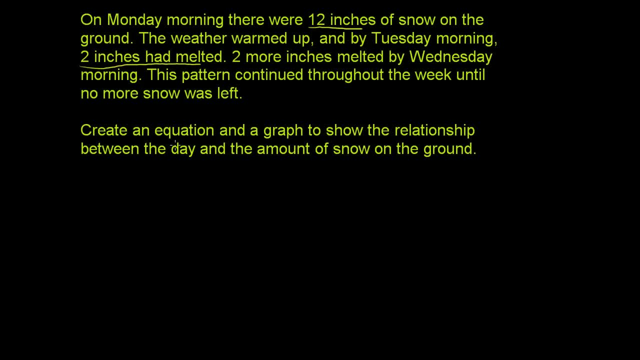 Wednesday you'd have 8 inches and that pattern continued. And what they say is: create an equation and a graph to show the relationship between the day and the amount of snow on the ground. So let's define a variable that tells us how far away we. 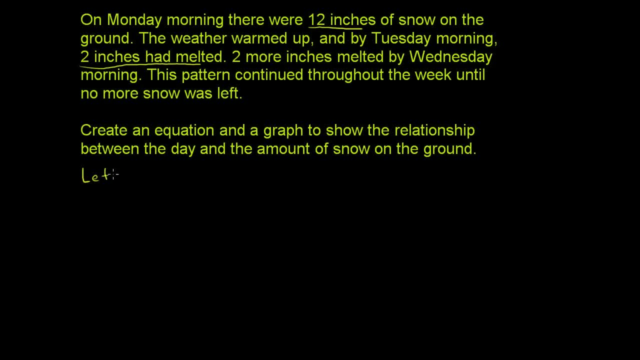 are from Monday. So let's let x equal to days after Monday, And then let y equal to days after Monday, So let y be equal to inches of snow on the ground. So one way to think about it is OK when x is 0, when we're. 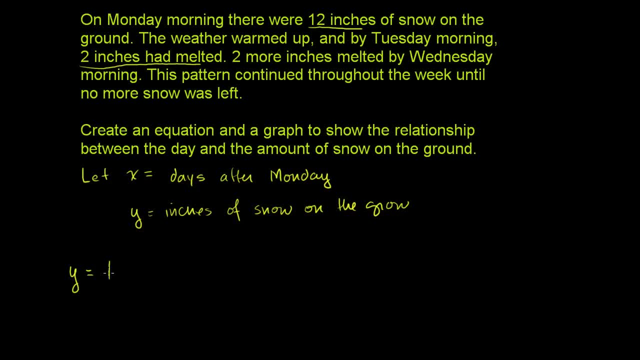 on Monday, when we're 0 days after Monday, we're going to have 12 inches of snow on the ground And then every day after that we're going to lose 2 inches. So if we're on Tuesday, On Tuesday we're going to have 2 inches times 1, because 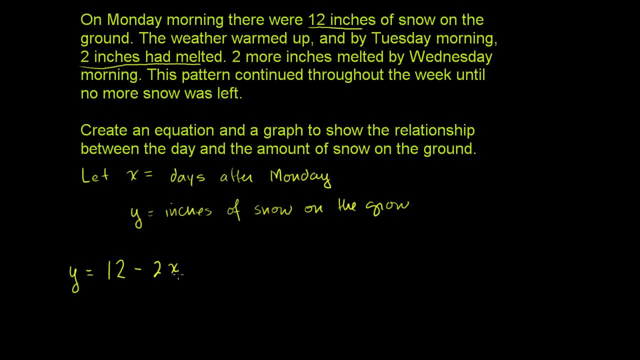 Tuesday is 1 day, So if x is 1,, that means we're on Tuesday. If x is 2, that means we're 2 times 2.. We've lost 4 inches, which is what the case is on Wednesday. 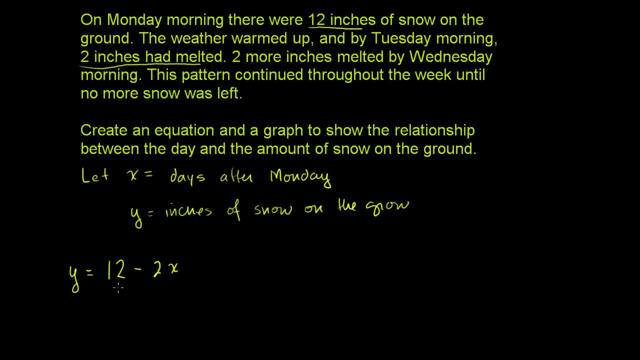 So this is our equation for the relationship between the day and the amount of snow on the ground: x is the day, how many days after Monday, And then y is the inches of snow left on the ground. So we start with 12, and then every day we 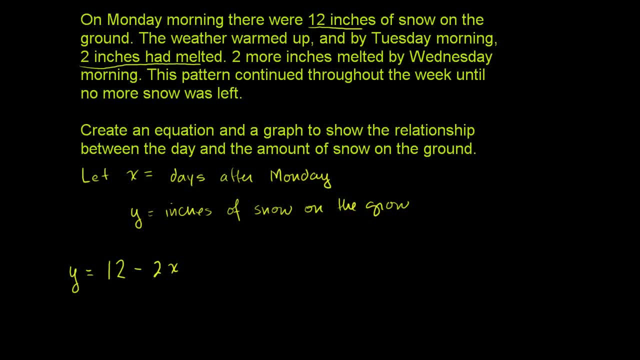 lose exactly 2 inches. Now let's graph this. Let's graph it. So I'll make my vertical axis the y-axis, That's inches on the ground- y is equal to inches left on the ground- And then the horizontal axis, that is our x-axis. 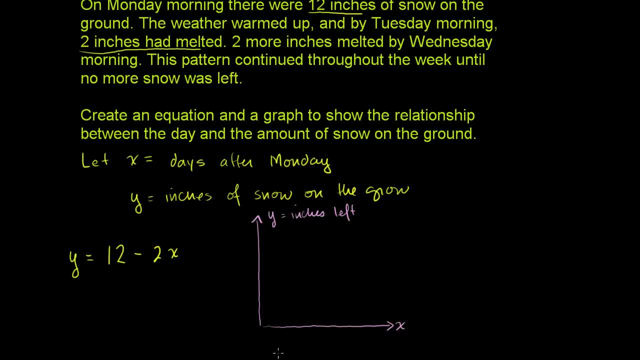 Let me scroll down a little bit. This is days after Monday, And so we have 0 days after Monday. We have 1,, 2,, 3,, 4,, 5, and 6.. And then on Monday, which is exactly 0 days after Monday, 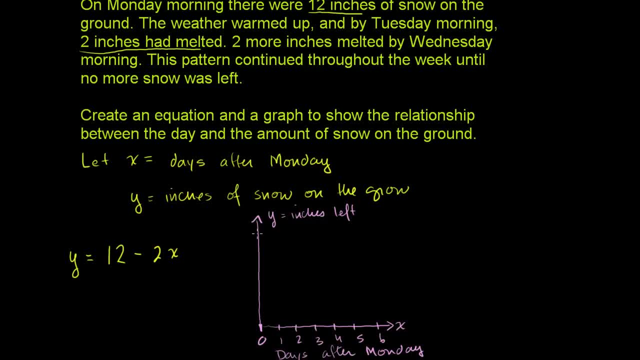 that is Monday. we have 12 inches on the ground, So I'll do it up here. So we have 12.. We have 12 inches on the ground right there And actually I could do a table. if you like, Let me draw this. 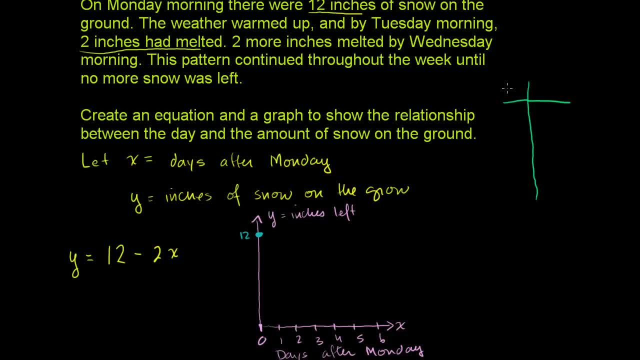 So if we do x and y, If you do x and y, this is the days after Monday. So 0, 1,, 2,, 3,, 4,, 5,, 6.. And then on the first day, we have 12 inches. on Monday: 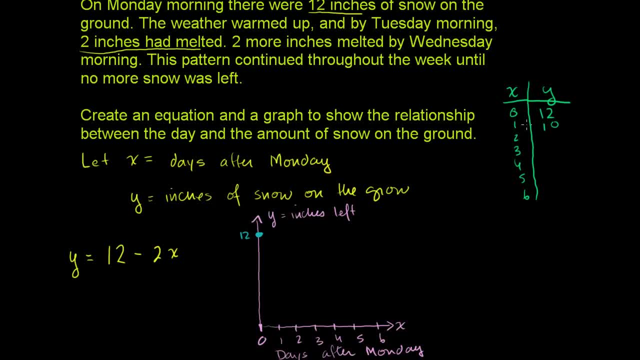 0 days after Monday. Then we lose 2 inches each day. On day 1, we have 10. Day 2, 8. 6. 4. 2. 0.. So let's plot these points. 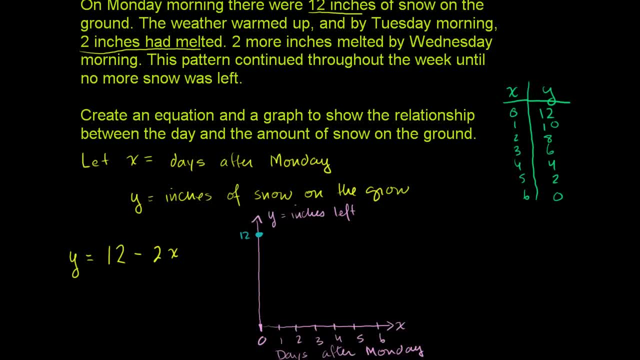 We already plotted 0, 12 in that blue color. Now let's plot 1, 10.. 1, 10 is right about there. It'll be right over there. Then we can plot 2, 8.. So 2 days after Monday, we have 8 inches left on the ground. 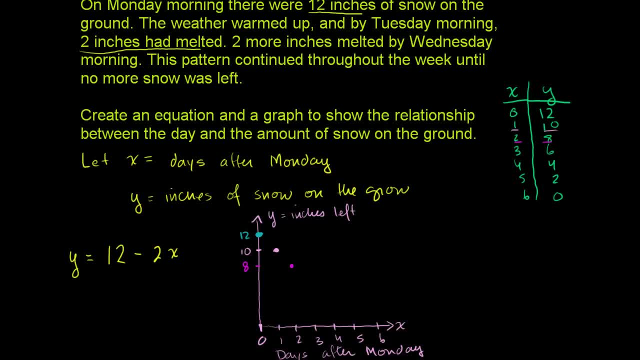 So this is on Wednesday, So that's 8 inches, And then on Monday, So that's 8 inches, And then on Monday, So that's 8 inches. So that's 8 inches. So we're at 3 days after Monday. 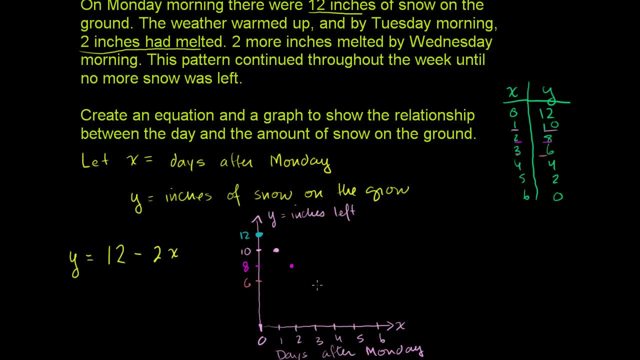 We've got 4 days and 3 days. So we have 4 days after 1 day after. So what a nasze? Now 5 days. Now write the numbers down: 1., 3,, 4.. 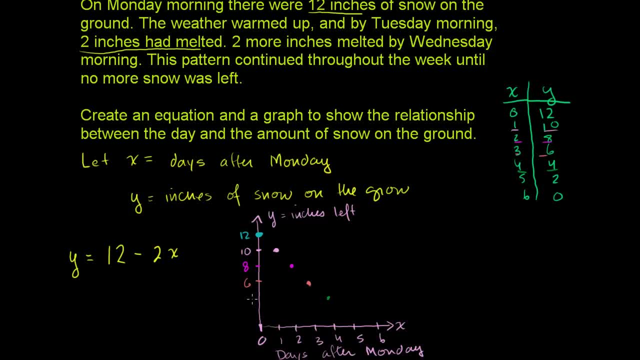 Week after week In your day. Week after week. Week seven, Week Nom evacuate is today. Week after week. Week after week, Week two, day, Week three In week three And then finally, on the sixth day, six days after Monday. 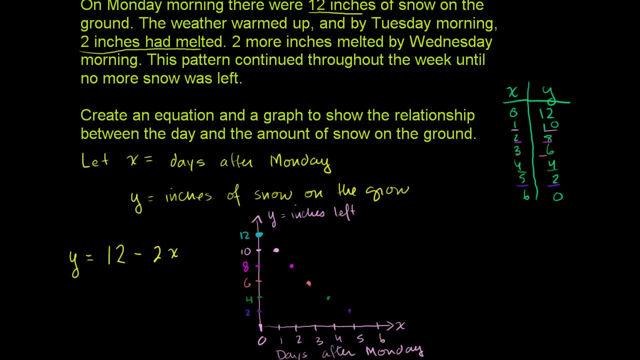 so what are we at Sunday? now? we are going to have no inches on the ground. So that's that, right there. And you can see that there's this line that formed because this is a linear relationship. It looks a little curvy because I didn't draw it. 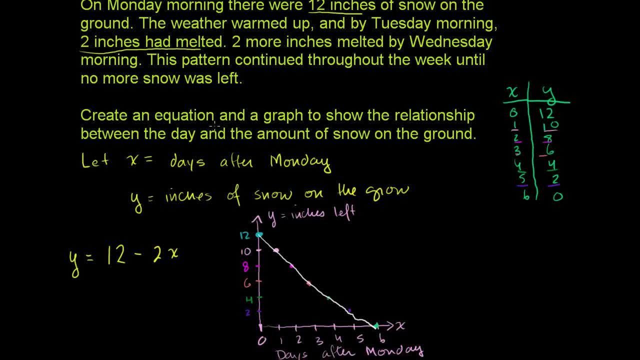 perfectly, but that is a line. So we've done everything. We've created the equation. We start with 12 inches Every day, after that we lose 2 inches, And we showed a graph that depicts the relationship. 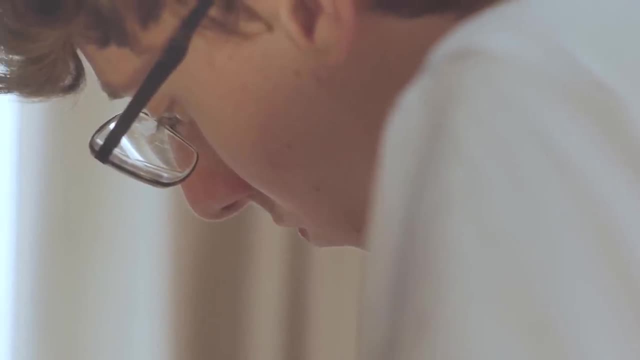 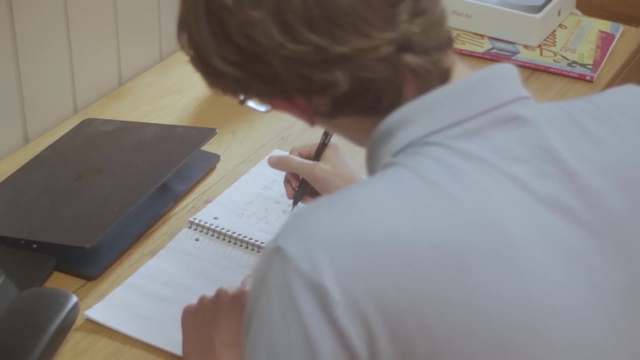 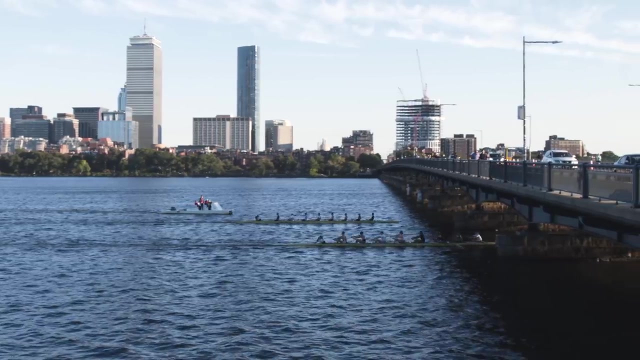 This problem somehow got under my skin. It seemed so obvious, yet it resisted all my attempts to prove it. It was just stubbornness on my part that I didn't want to take no for an answer, So I kept going. To me, math is really about connections between things that seem totally. 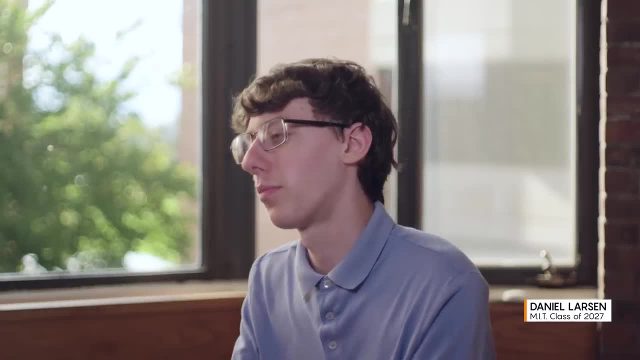 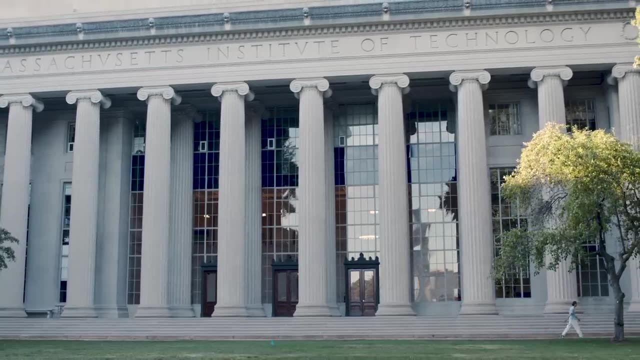 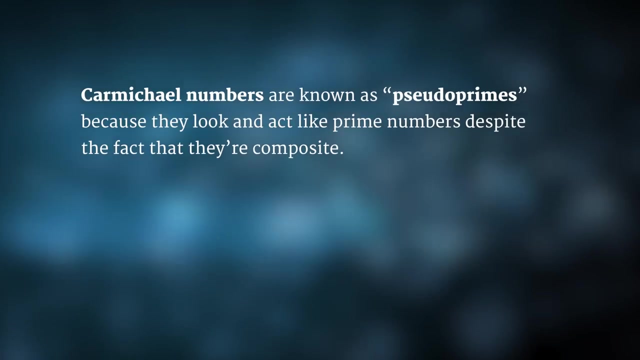 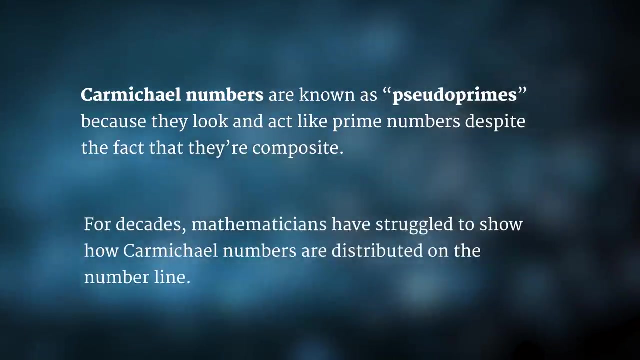 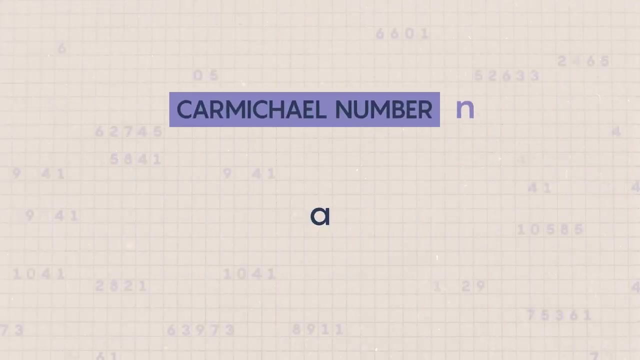 unrelated and it's sort of always there for you. My name is Daniel Larson, I'm a freshman at MIT and I'm studying mathematics. When I was in high school, I got interested in Carmichael numbers. A Carmichael number is a number n, such that for all integers, a a to the n minus a. 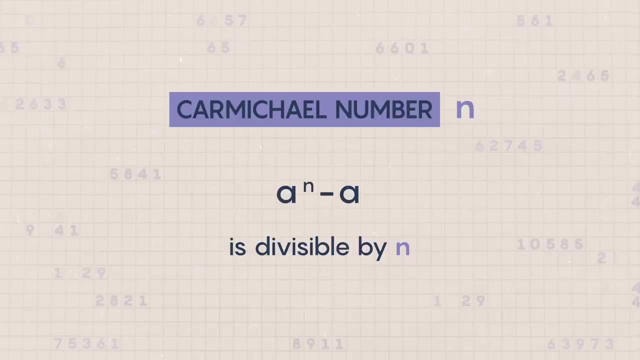 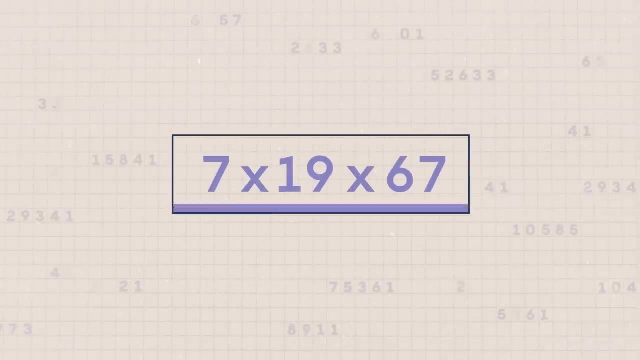 is divisible by n, And furthermore, this is where it gets interesting: n equals n And n is not prime. So the way you construct Carmichael numbers is you build them out of prime factors which have a special property. But the problem is it's. 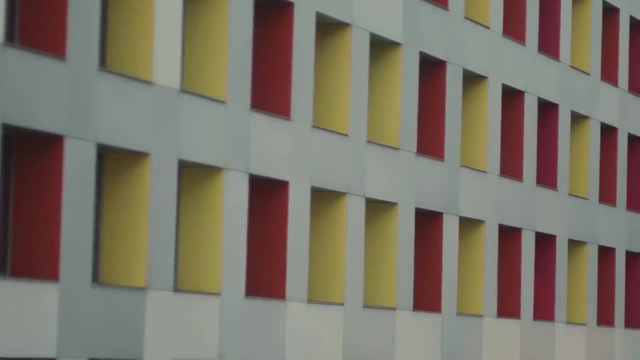 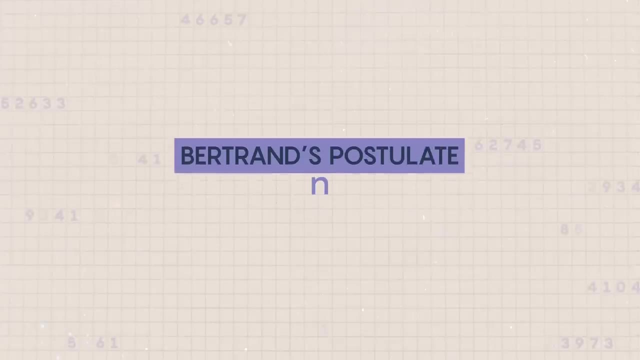 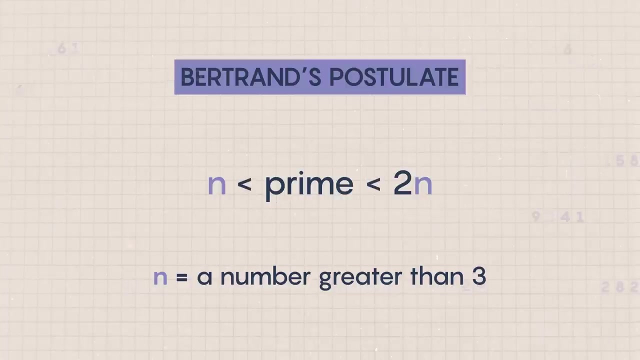 difficult to say in advance how many prime factors these numbers will have. without knowing how many prime factors they have, it's difficult to get an exact read on the size. Bertrand's postulate for primes says that for every large number, there exists a prime between that number and its double, And so we would like to.